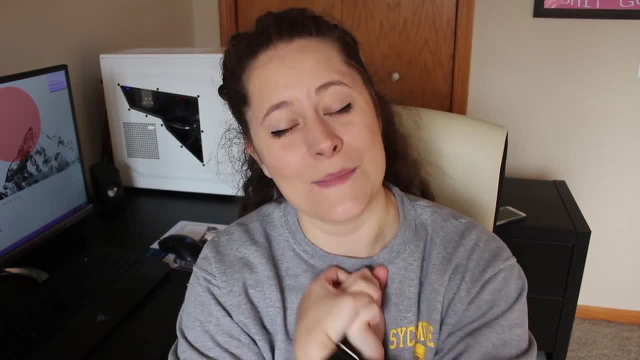 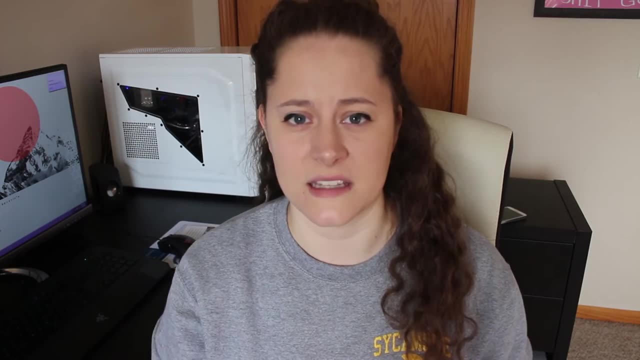 Then that's a very tall order. when it comes to fossils, We have to remember that the creation of fossils is an unlikely event. The environment and the factors that go into fossilization have to be just right for it to even occur. And even if you do become a fossil, there's a good chance that you're going to be destroyed. 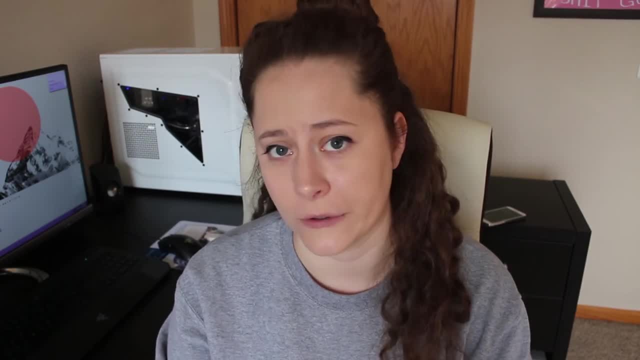 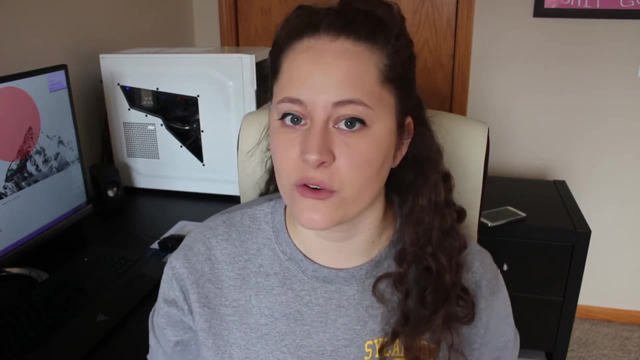 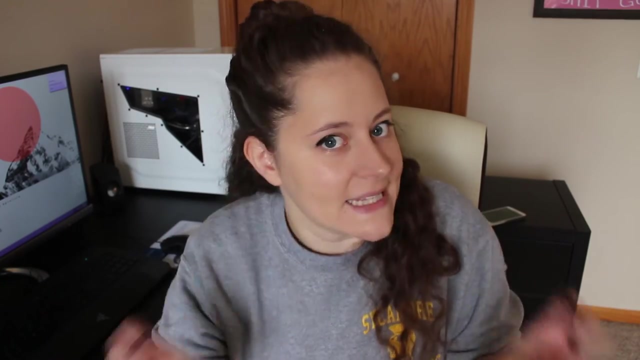 before a sentient ape evolves and picks you up and decides to categorize you. And, lastly, there's an awful lot of geologic strata that we cannot see. It is below us and will likely never reach the surface. So, because the fossil record is incomplete, there's always a lot of talk about finding the missing link. 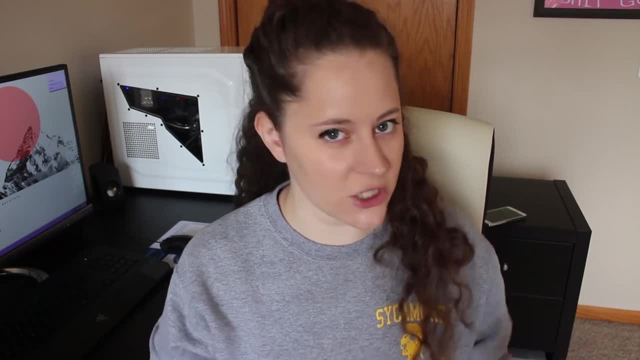 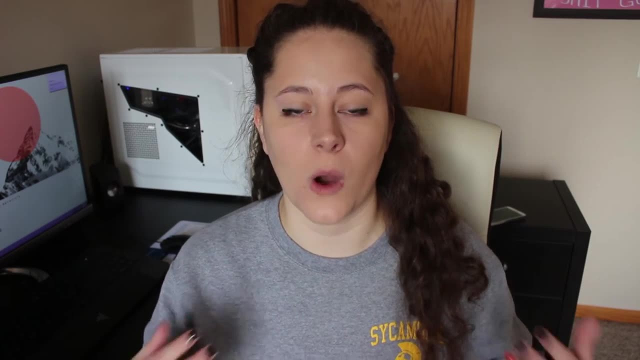 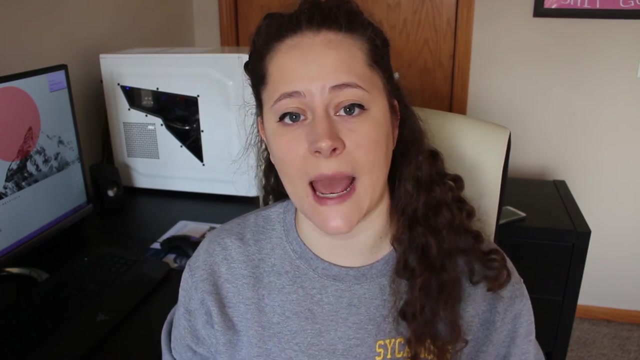 And what most people mean by missing link is simply a transitional form between two branches of evolution. One missing link or transitional form is simply going to open the doorway to other transitional forms with smaller changes. It is also important to remember that any transitional species is going to happen in a small population. 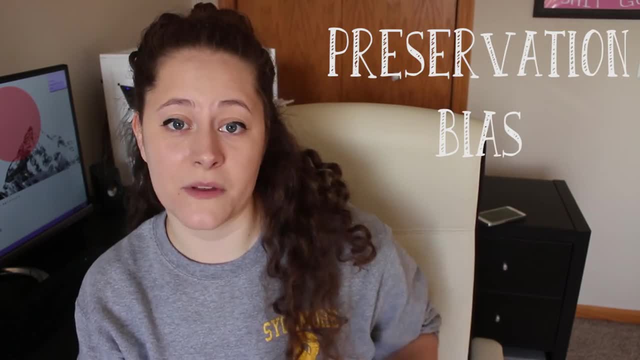 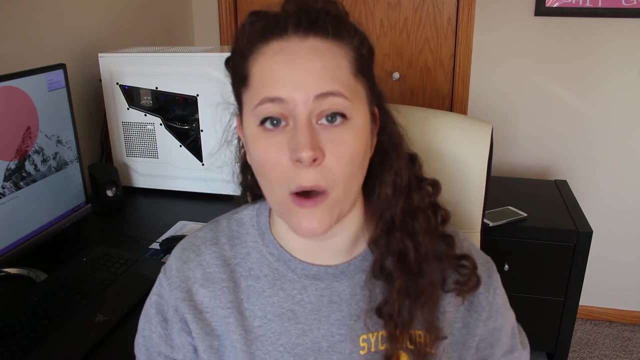 And if we remember some terminology, then we should remember that the more of you there are, the more likely it is that you will become a fossil. However, there is one story that I wanted to share with you guys about the discovery of a so-called missing link, or a transitional form. 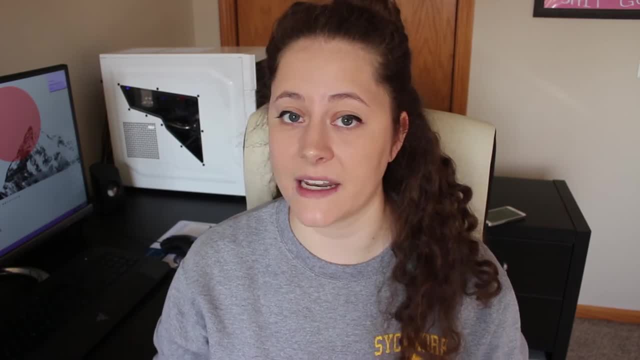 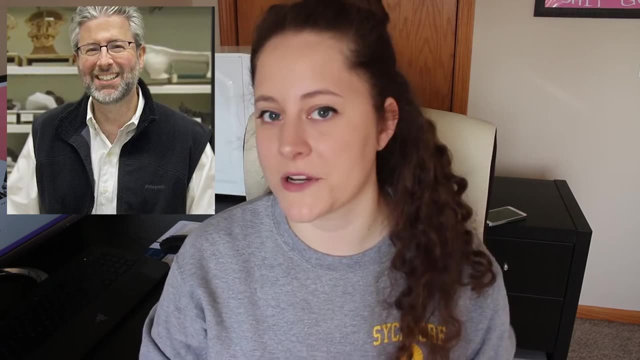 And that is the transition between a vertebrate that was adapted for land and the ones that were adapted for water. These transitional fossils were discovered by somebody named Neil Shubin in the very northern part of Canada. Shubin's team found a pit of fish skeletons that were so well preserved. 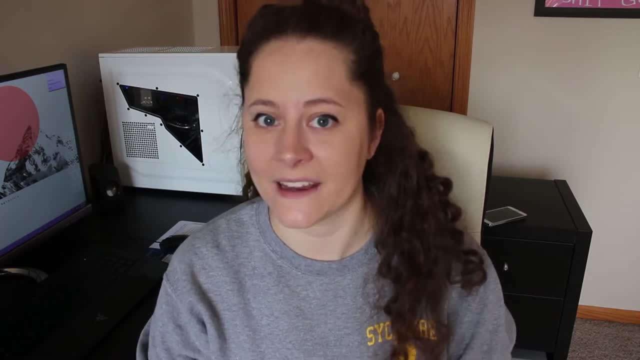 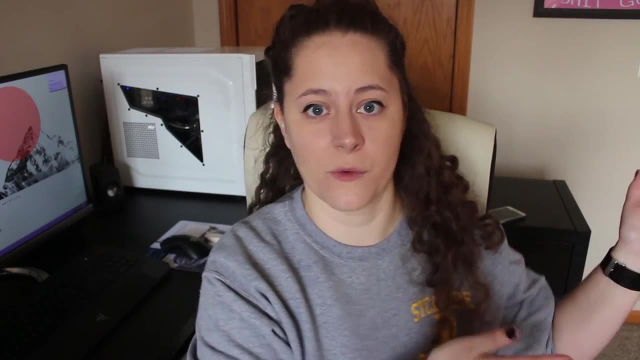 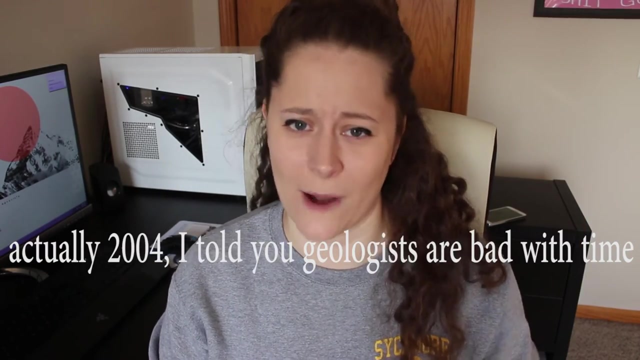 that they were able to determine that this was the missing link between vertebrates that were adapted for water and those that were adapted for land. They basically split these adaptations right down the middle. Half were very water-based and half were land-based. This was in 2006,, and that is like basically an hour ago to geologists. 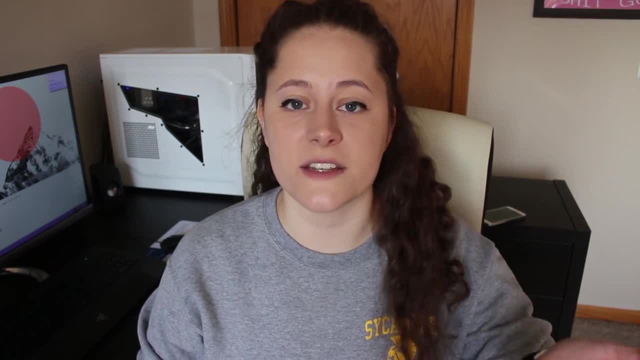 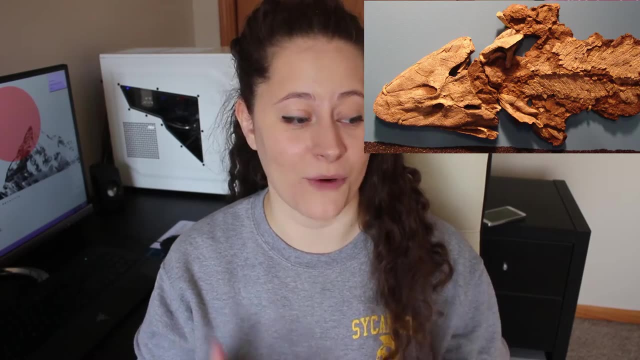 This creature was characterized as a lobe-finned fish and I would be surprised if you guys haven't heard the name, because the name is Tiktaalik And I feel like it's such a unique name that we probably remember it when we hear it. 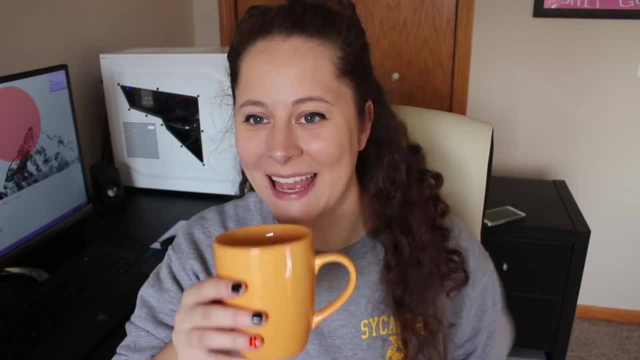 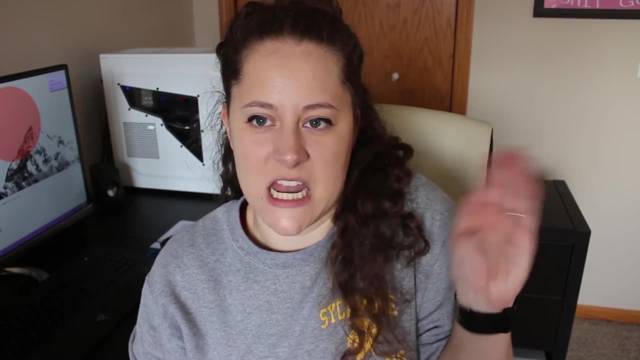 Tiktaalik. I love it. It's so fun to say This wasn't the first Tiktaalik to be found. We found another one in 1998.. This was the first Tiktaalik because it was just a fin and it had finger-like digits forming.